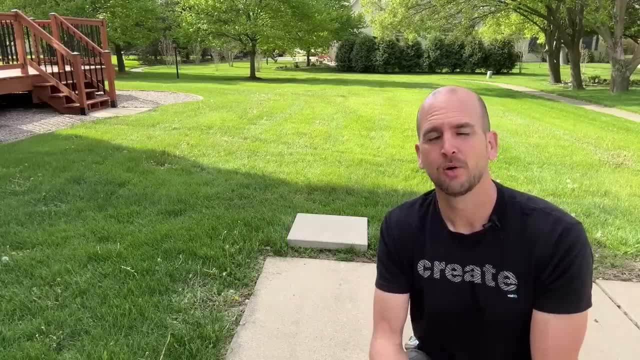 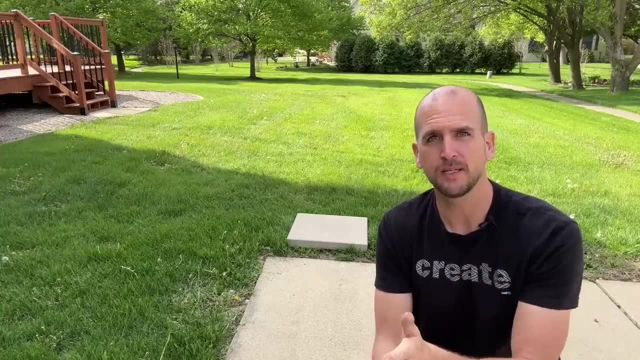 some of your other options, like pouring a concrete sidewalk or laying down some kind of gravel path. This is a great solution to get you a more defined walking path to a garden bed, maybe a seating area along your landscape or, like me, from your driveway over to your deck. Now I need to run. 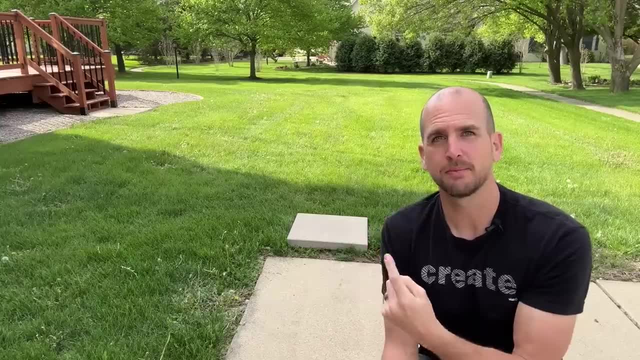 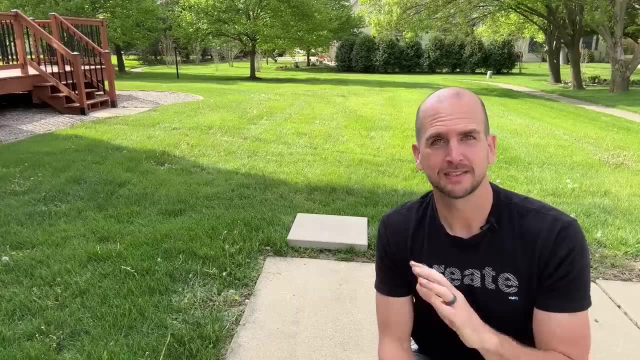 about 24 feet between my driveway and my deck, and I'm going to be using simple pavers, like the one behind me, which are just a square about 20 inches by 20 inches. But you can use this exact same application if you want something a little more natural or if you even want to go into the high. 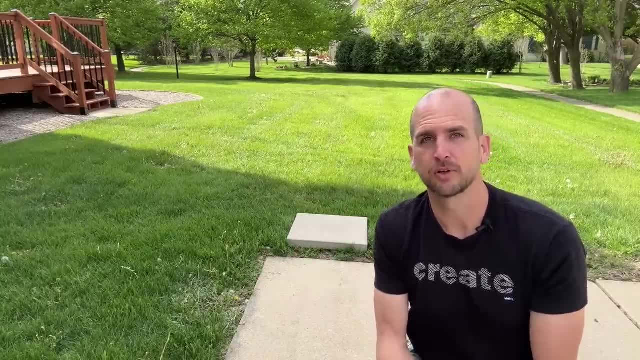 end like flagstone and get a really great look for your lawn. So, first up, I'm just going to start laying out those pavers and get my pattern set and then we'll start integrating them into the lawn. So I'm going to start laying out those pavers and get my pattern. 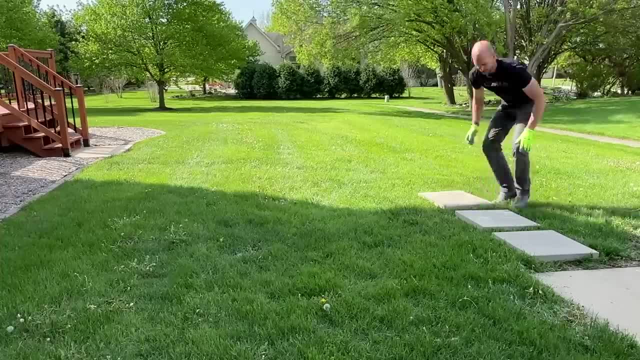 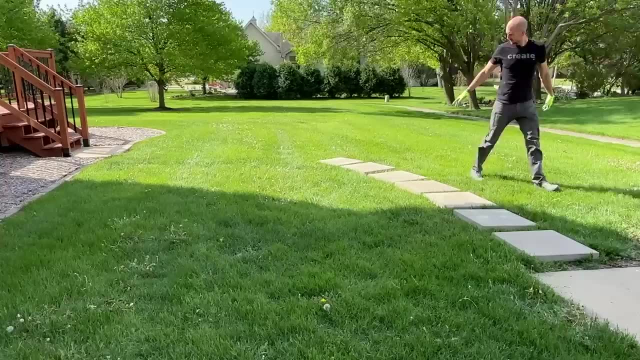 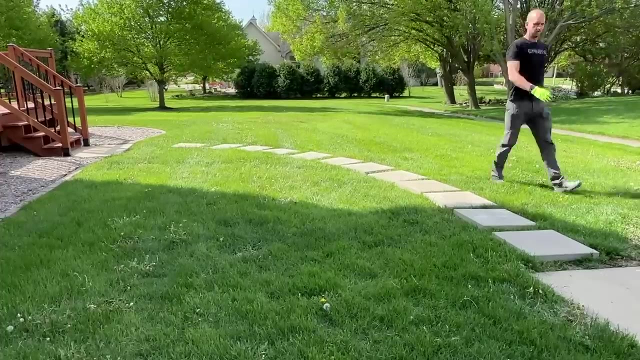 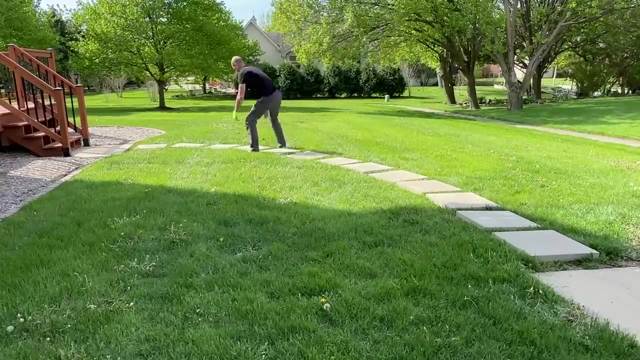 set and then we'll start integrating them into the lawn. So first up, I'm just going to start laying out those pavers and get my pattern set and then we'll start integrating them into the lawn. So just laying them out. There's no pressure here. You got time to move those around. You're going to kind of be able to play with your pattern. I'm just doing a simple arc, so it's not that complicated. There's going to be 13 pavers and these are fairly large- 20 by 20 inches- and they weigh about 55 to 60 pounds per paver. So they do have a little weight to them, which can be a good thing from stability, but also is a little bit to haul around. So here is what the pattern looks like. 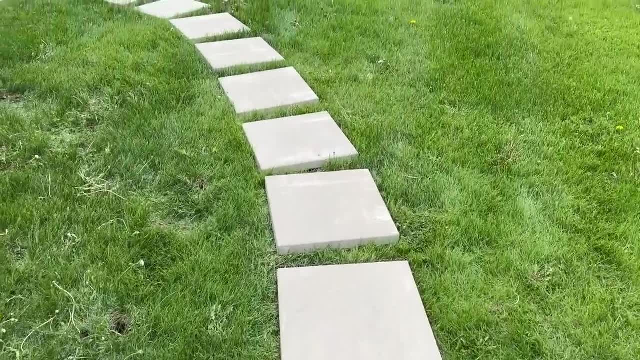 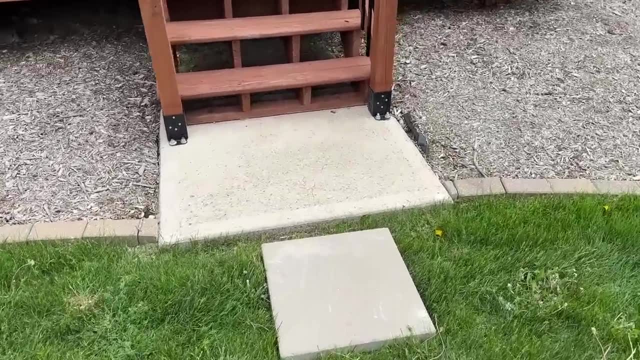 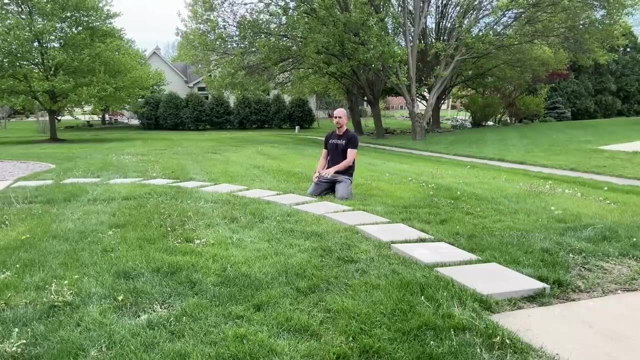 path looks like we have an arc all the way along, but we do kind of get a little more aggressive with the curve here at the end once we get close to the landing pad itself. now, what i really like about the paverstone type of project is you can get everything set in place. you can really see. 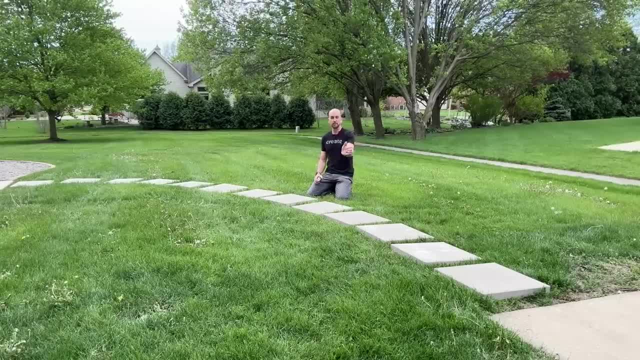 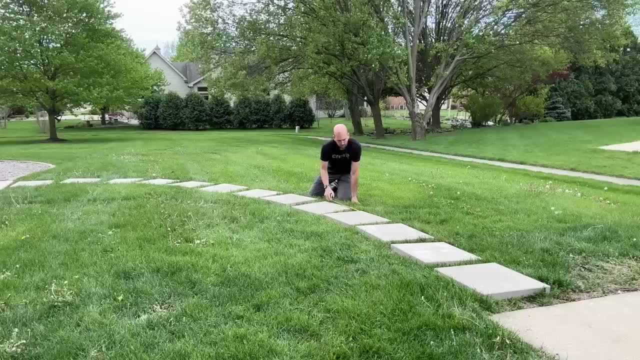 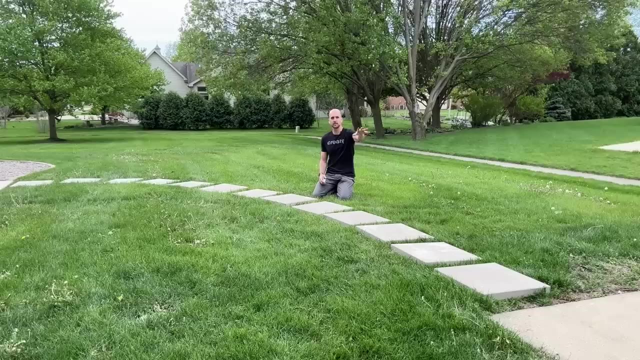 your design, see how it looks, make changes. make- maybe you're making a winding path, so you're going to keep changing that around. take some measurements, making sure you are consistent with your spacing along the path, and then make any final adjustments before we start actually cutting around these and then setting those flush with the ground surface, which is what we're going. 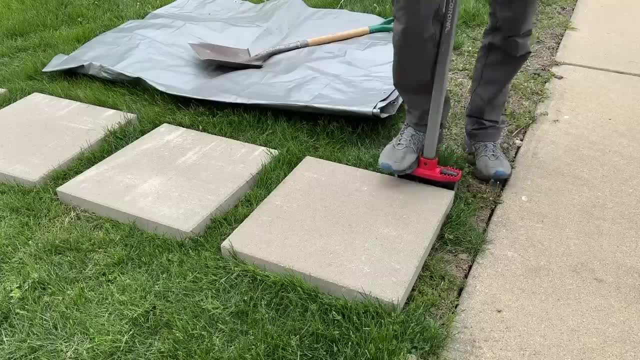 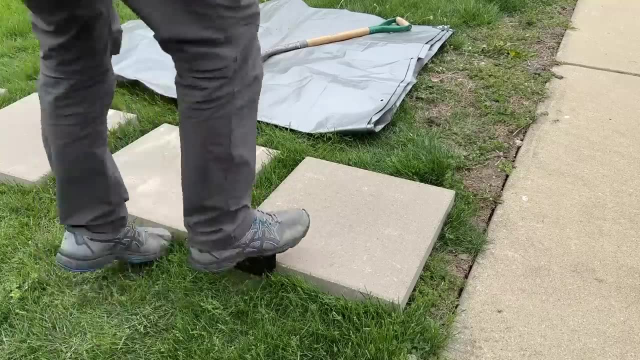 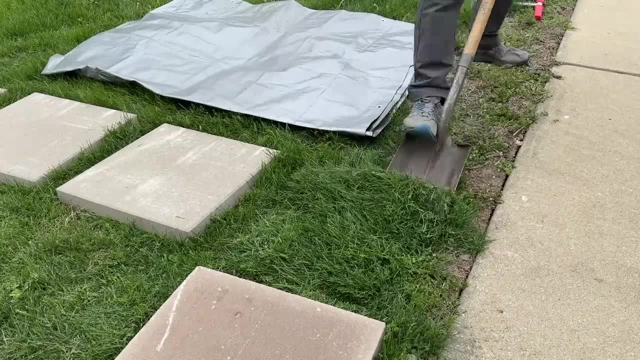 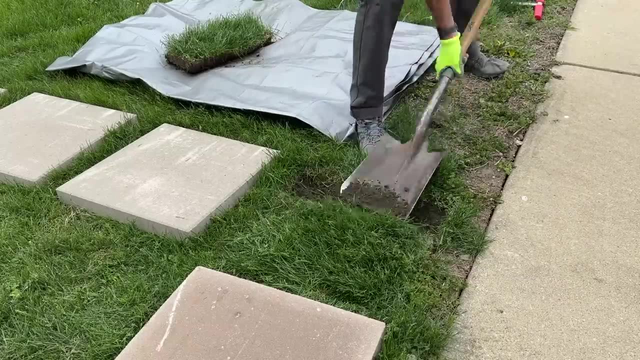 regular flagstone. it'll come in super handy. then we'll just go ahead and take up the sod. you can take it up in one big piece or just multiple pieces. i like to use a little tarp because i'll drag that sod over. and don't forget, you can use that sod in other parts of your yard. 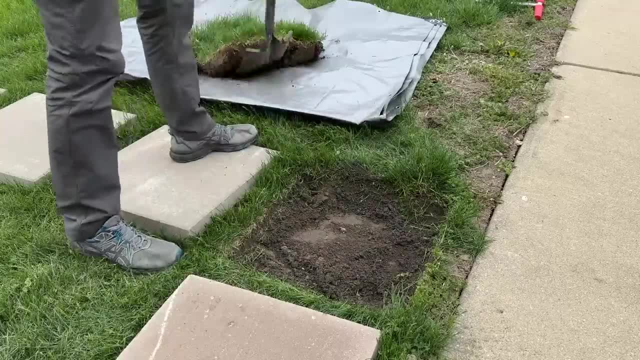 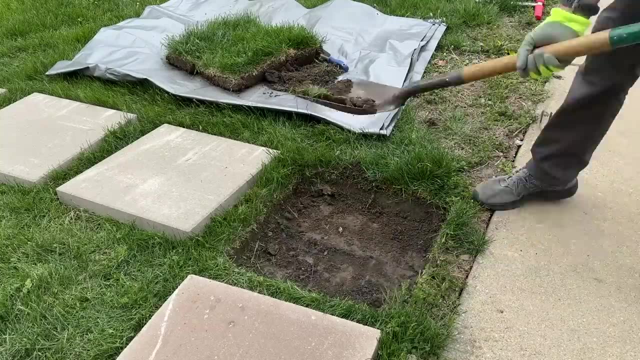 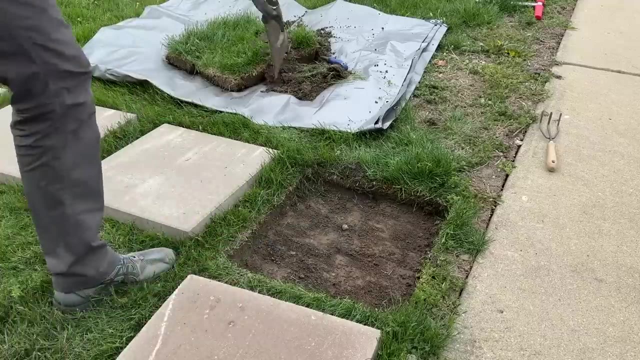 like that part there where you can see it's having trouble growing grass, i can kind of transplant that right in that space as well to get the grass going. then we'll clear things out and kind of measure up how deep this is. the old overall depth right here is about three inches and the depth of our paver is about two inches. 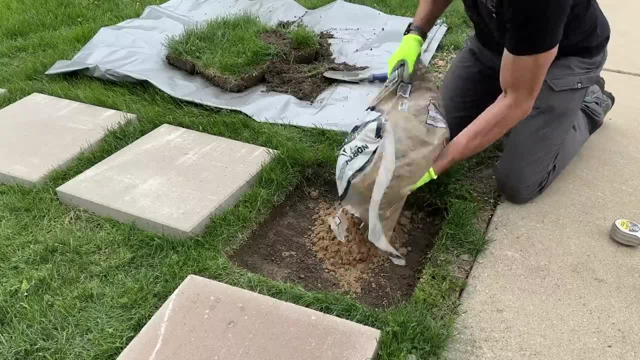 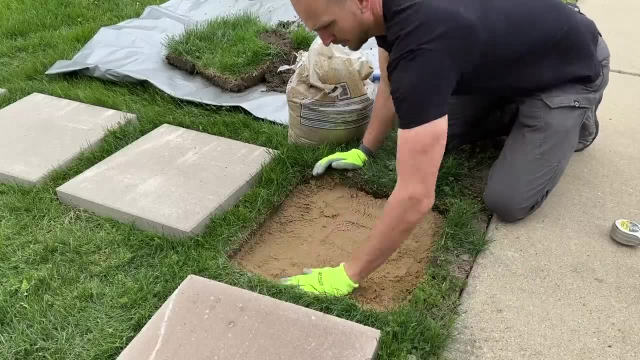 so that's great because now i can lay down some sand to give it a much better base. nothing fancy here, just basic paver sand and we'll level that out, fill into the different corners, and sometimes you'll have to do multiple different trials here and measure out to make sure you have. 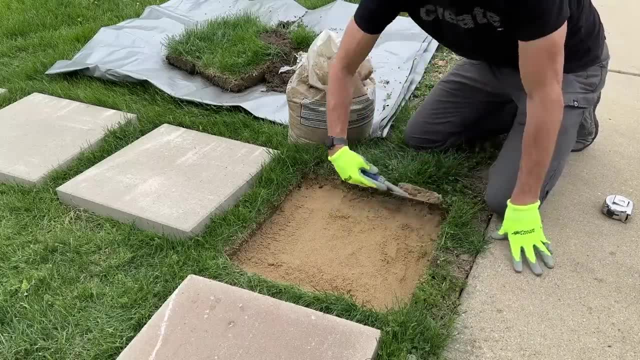 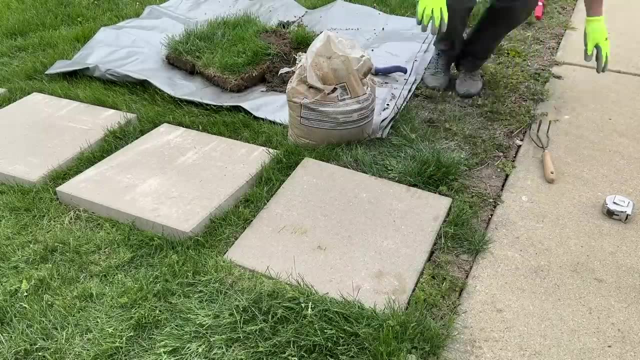 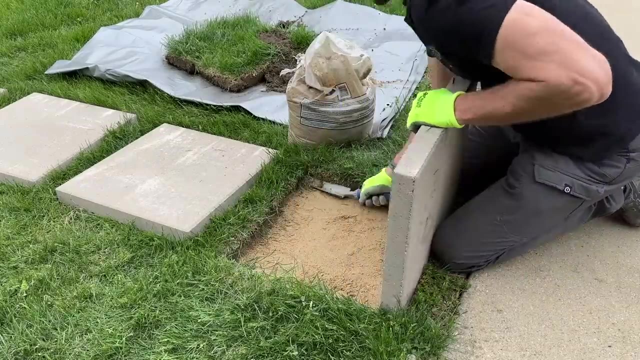 the depth correct and that you have a nice solid foundation and no like teeter-tottering when you put the paver into space. so once you're set you can flip that into space. if you have a little bit of interference after you knock it around with a mallet, then you can make adjustments, taking a little material out. 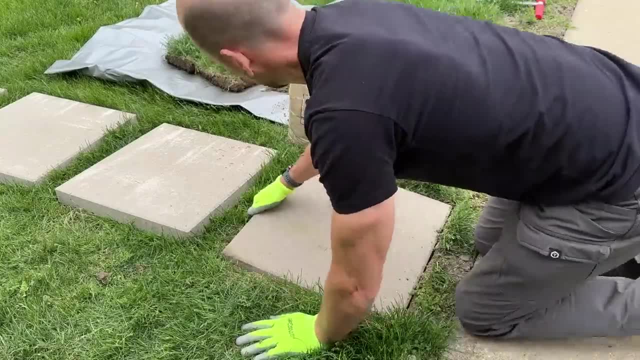 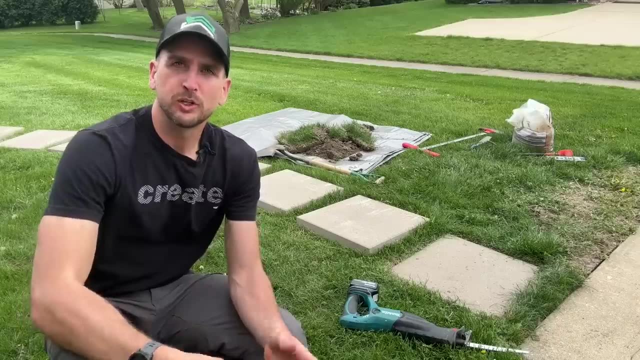 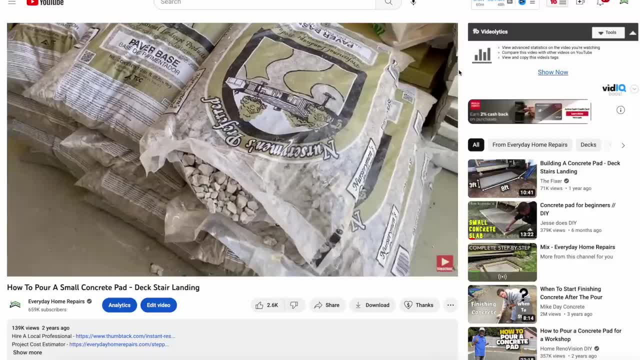 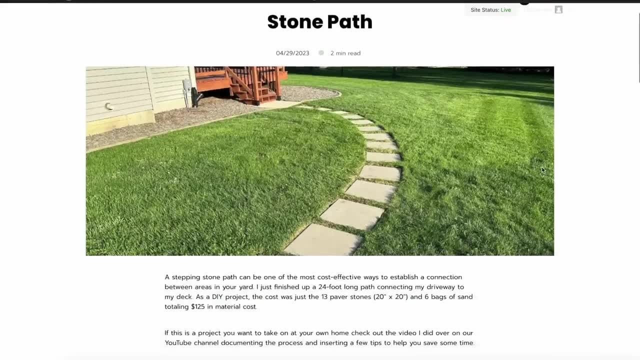 I'll finish off this project, but also below the video you'll see a link to a page that I put together which is going to help you estimate the cost if you hire this out. So I'll look at different labor rates and then show you the material cost so you get a better idea if you're 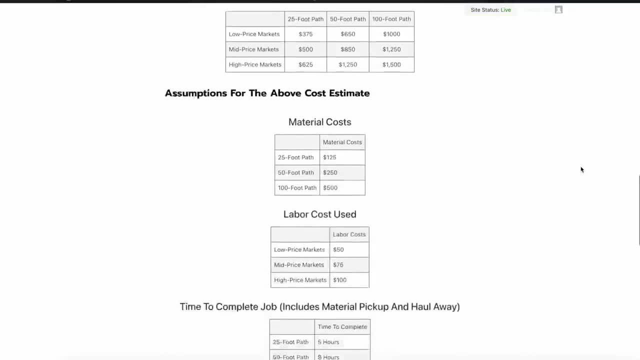 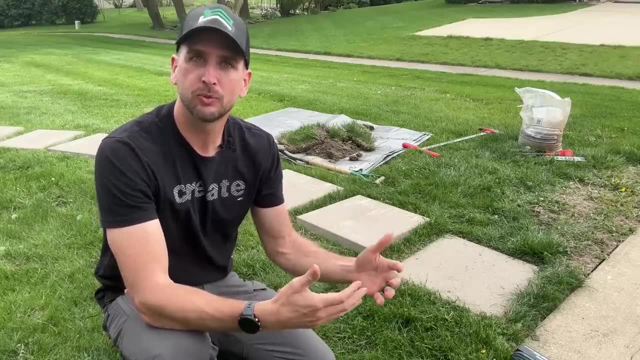 not going to do a DIY, which we'll talk about that cost. what are you looking like in terms of cost hiring that out? Then, after looking at those costs, if that's something you want to go forth with, we are also getting a nationwide network of professionals to help you out. so from that link, 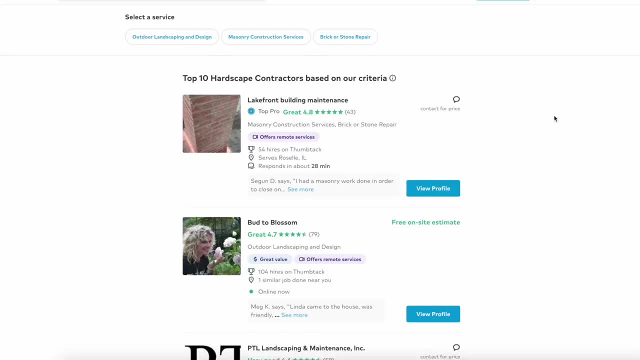 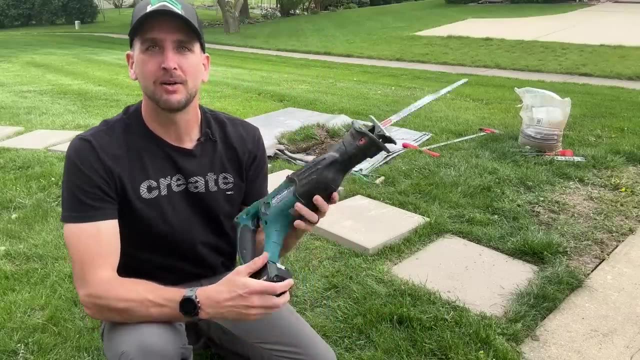 we'll send you over. you can select landscaper, give a little more details on your project and then get rolling and get that accomplished and off your to-do list. But if you are doing this DIY, let's jump in and show how actually a sawzall is pretty handy for cutting around each one of these pavers. 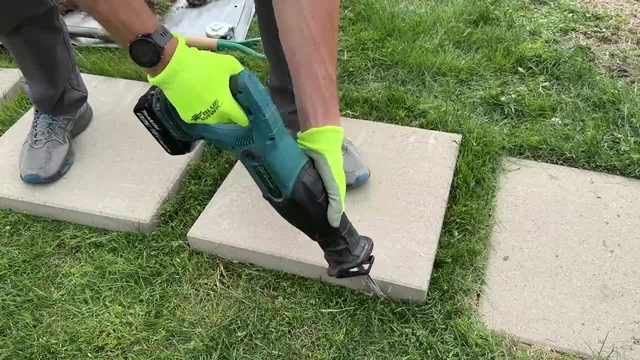 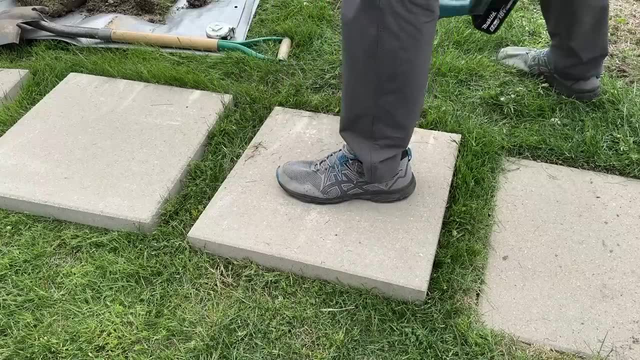 to get them inset into the ground. Now I just have a longer wood blade, but obviously you don't need any specific blade here. it can be rather dull. I like to do a little bit of a sawing motion. I let the blade do most of the work, but I saw it back and forth at a slight angle. 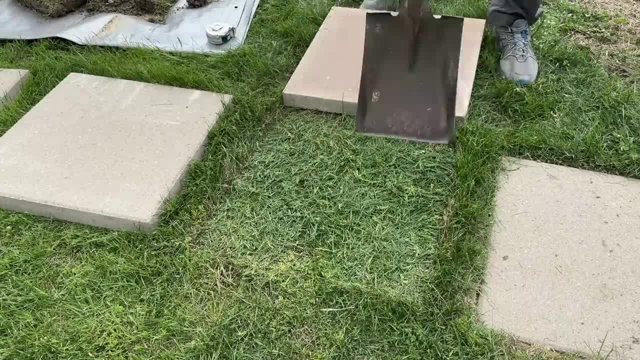 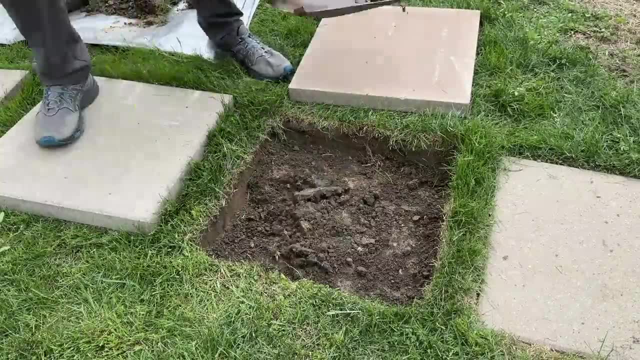 so it doesn't get caught up on things like dandelion roots, and then you'll use that same spade, we'll work up that side again one piece or multiple pieces, and then cut things down. Now, depending on if you want your pavers to actually be level, you should be getting your. 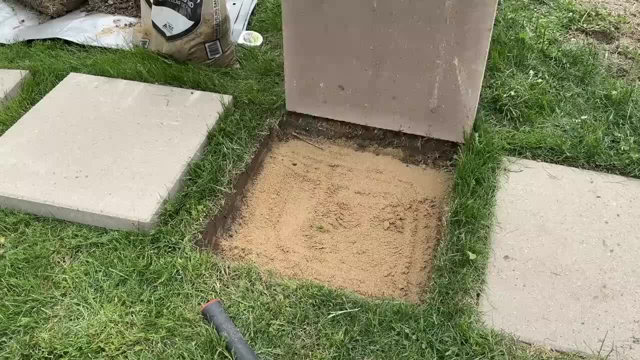 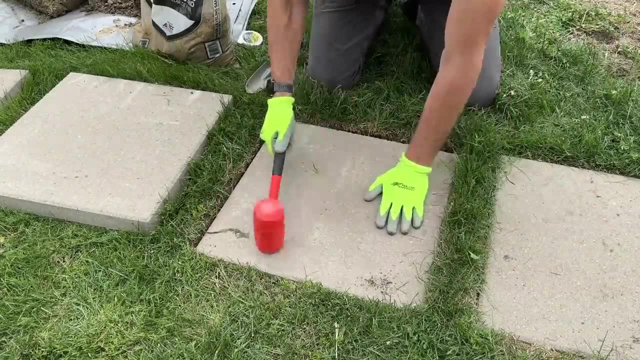 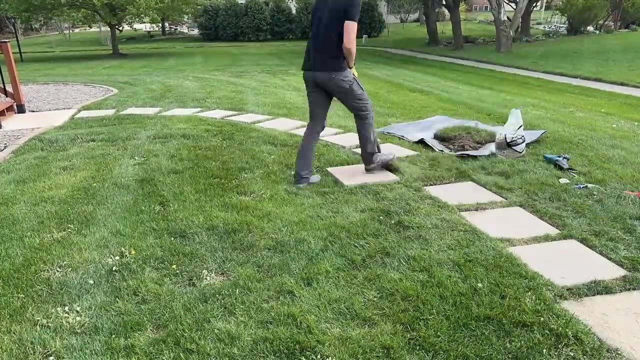 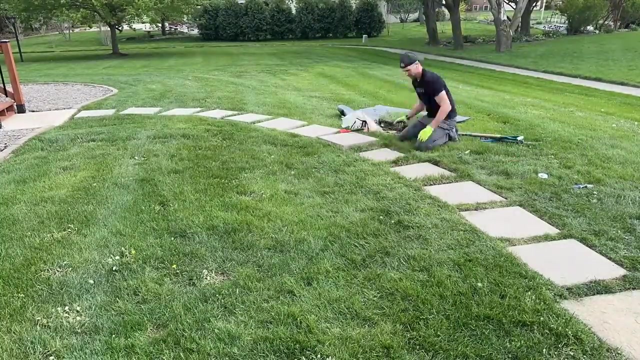 torpedo level out or something making sure all that sand's leveled up, or, like me, if you're more following the construction process, So I'll go ahead and continue to progress through this. to give you an estimate on cost, So I have 13 of these 20 inch by 20 inch pavers and I got about six bags of sand All in my material cost. 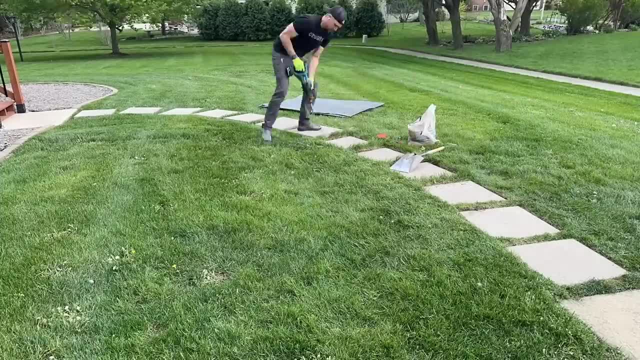 for this project is about $125, so really not that bad at all. Now, depending on if you get a lot fancier with your pavers, that material cost is going to be a little bit more expensive. So I'm going to go ahead and do that, and I'm going to go ahead and do that, and I'm going to go ahead and.